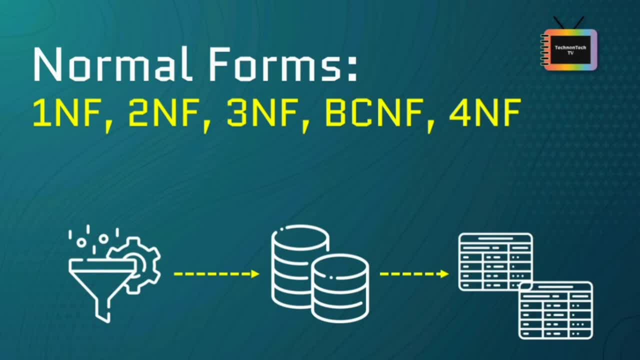 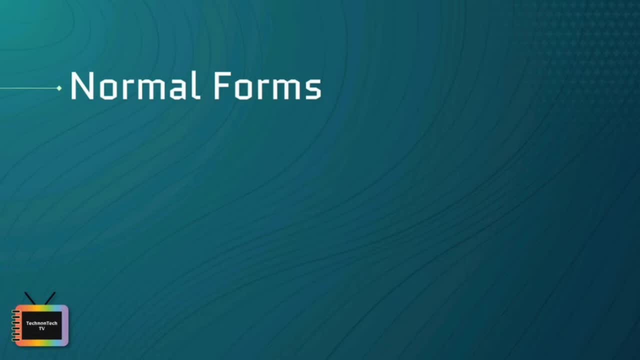 I will be going to discuss about different normal forms in DBMS. So let's start. So first understand what is normal forms. The process of normalization involves applying rules to a set of data. Each of these rules transforms the data to a certain structure called a normal form. 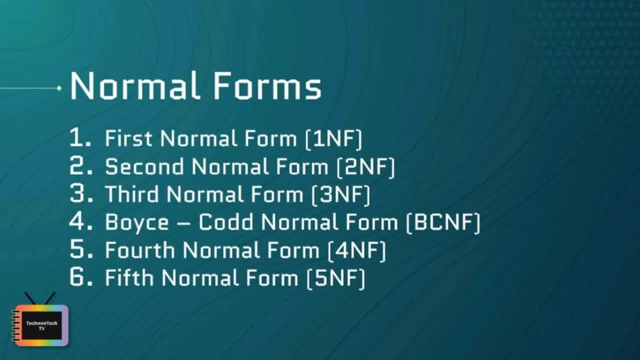 So there are total 6 normal forms, but there are only 5 normal forms which are commonly used. 5th normal form in database: normalization is generally not implemented in real-life database design, So in this tutorial we will cover 5 normal forms. So let's discuss. 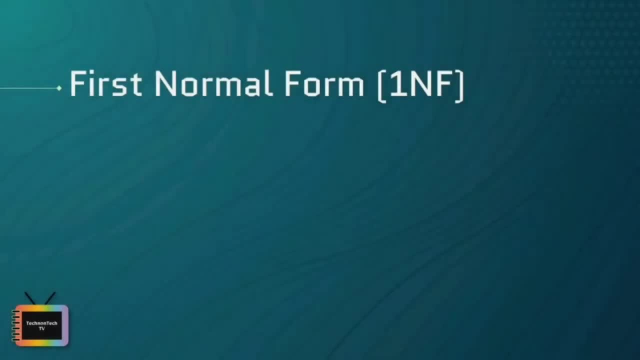 it one by one in detail, with examples. So first we have first normal form. A table is set to be in 1NF if it should satisfy 4 conditions. First is columns must have single values. It means that each column of your table should 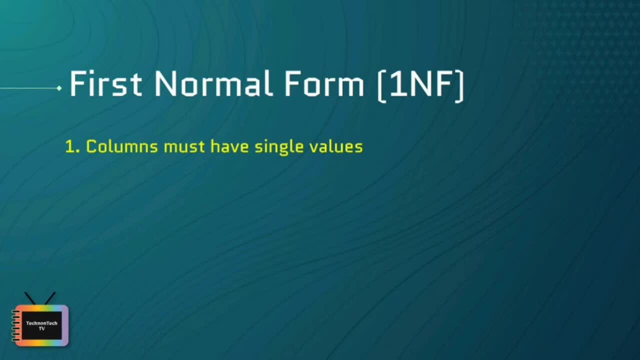 be single-valued, which means they should not contain multiple values. We will explain this with the help of an example later, So let's see the other rules for now. Second is: columns must have unique names. This rule expects that each column must have unique names. This rule expects that each 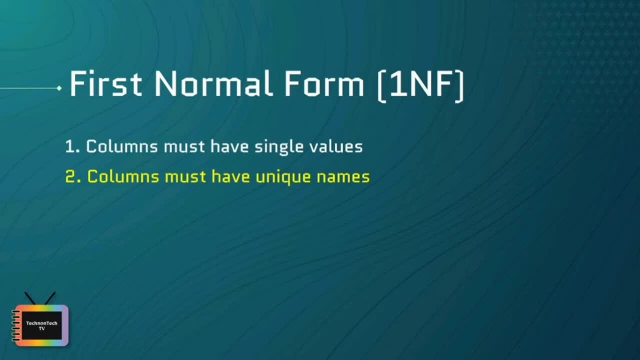 column must have unique names. This rule expects that each column must have unique names, So each column in a table should have a unique name. This is to avoid confusion at the time of retrieving data or performing any other operation on the stored data. If one or more 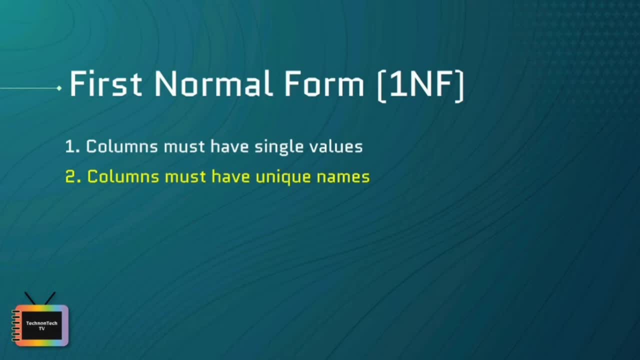 columns have a same name, then the DBMS system will be left confused. Now, third is values of a given attribute must be of the same data type. This is more of a common sense rule. In each column, the values stored must be of the same kind, So each 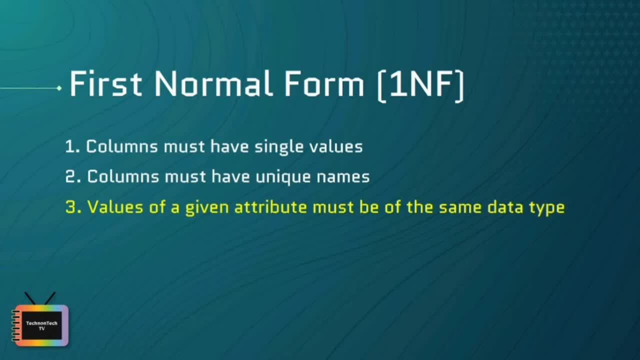 column must be of the same kind or type. For example, if you have a column dob to save date of birth of a set of people, then you cannot, or you must not save names of some of them in that column along with date of birth of others in that column It should. 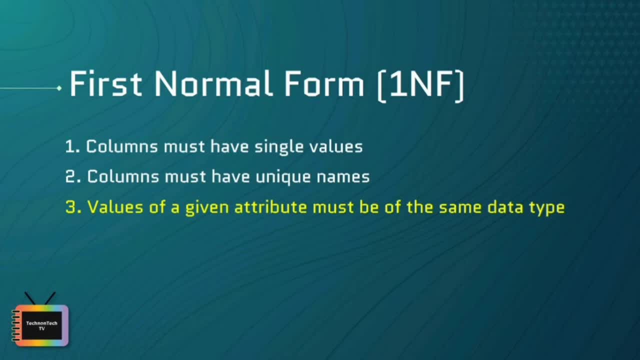 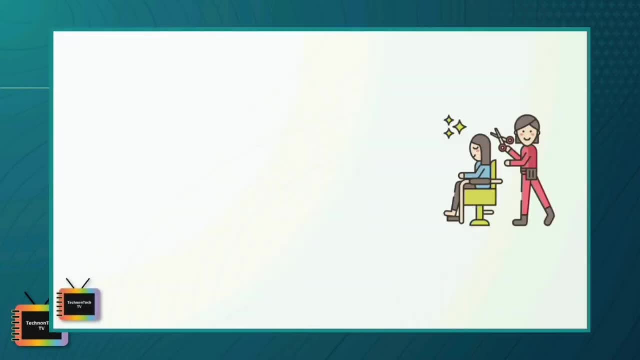 hold only date of birth for all the records or rows. Last is no two records or rows can be identical. Let's assume you are the new hairdresser in town and you want to store the names and contact details of clients in a database And your trainee staff creates this client info table. 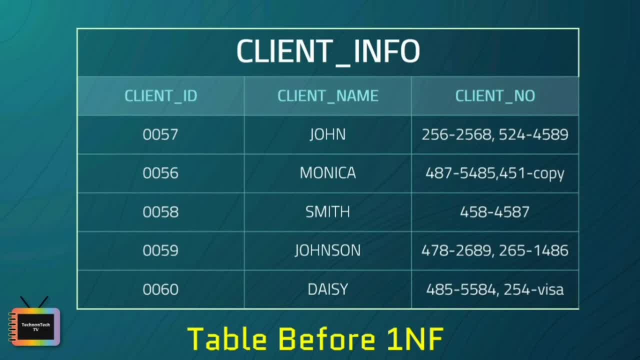 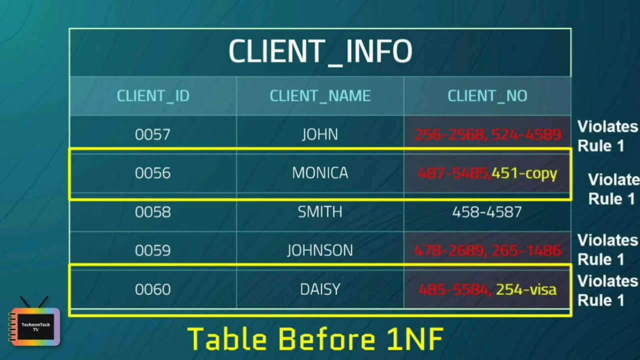 Look closely and you will see that the table does not conform to the rules of 1NF. The reason for this is that the trainee staff saved the second mobile numbers of John, Monica, Johnson and Daisy within the same field, which violates rule 1.. And the second entries for Monica. 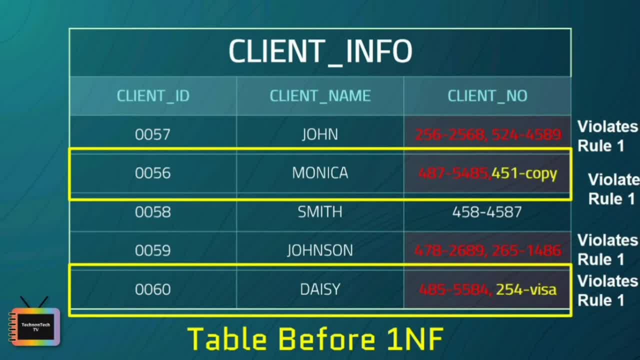 and Daisy are stored in wrong data format. The numbers are saved in number format, while the second numbers are stored as the string with numbers and letters, which violates rule 3.. So to avoid all this problem, let's apply 1NF rule in this table. So, after applying 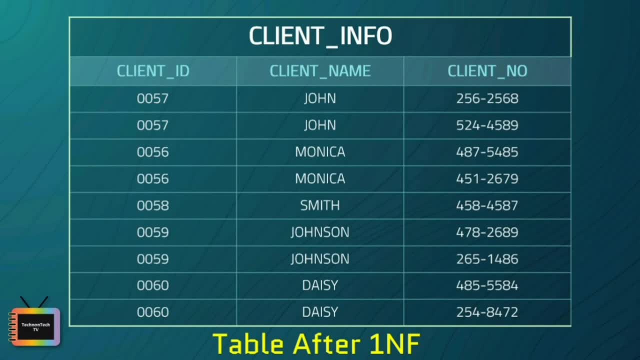 1NF table will look like this. By doing so, although a few values are getting repeated, but values for the client number column are now atomic for each record or row, So using the first normal form, data redundancy increases as there will be many columns with the same data in multiple. 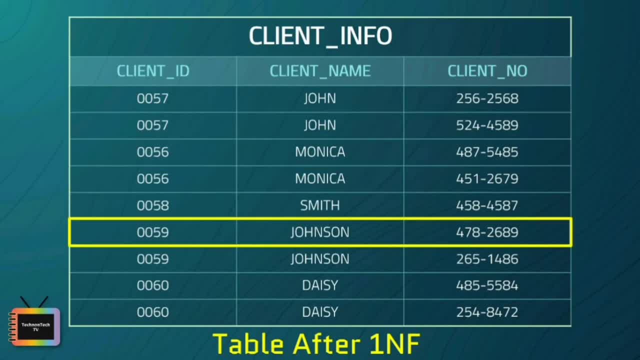 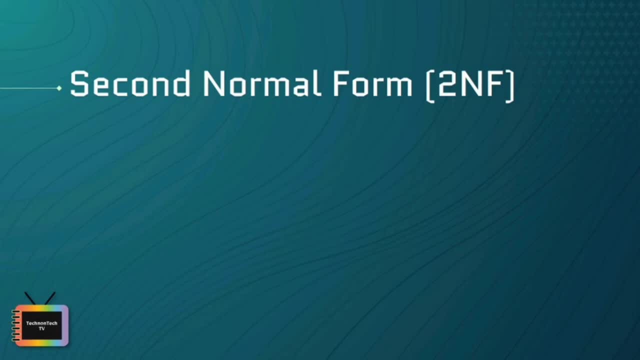 rows, but each row as a whole will be unique. Next is second normal form, or we can say 2NF. So for a table to be in the second normal form, it must satisfy two conditions: The table should be in the first normal form and 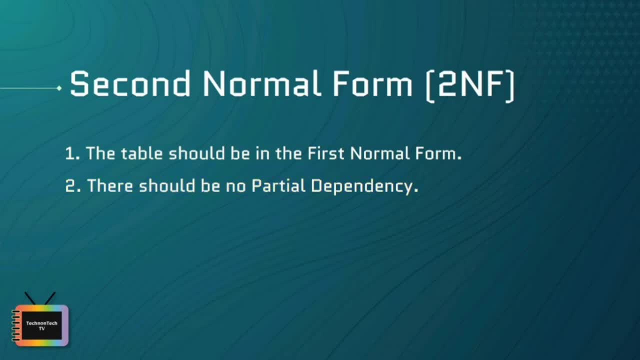 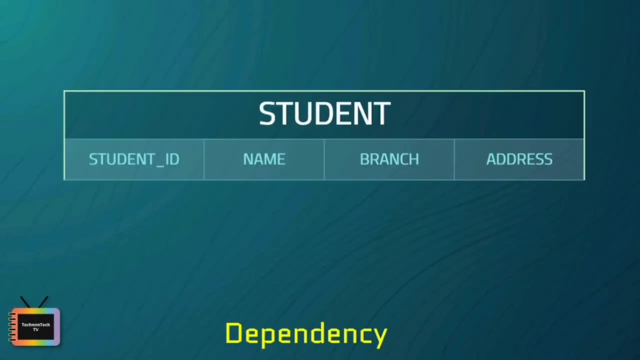 there should be no partial dependency. So every non-key attribute is fully depend on the primary key. So what is partial dependency? Do not worry about it. First let's understand what is dependency in a table. So let's take an example of a student table with columns student id name, branch and. 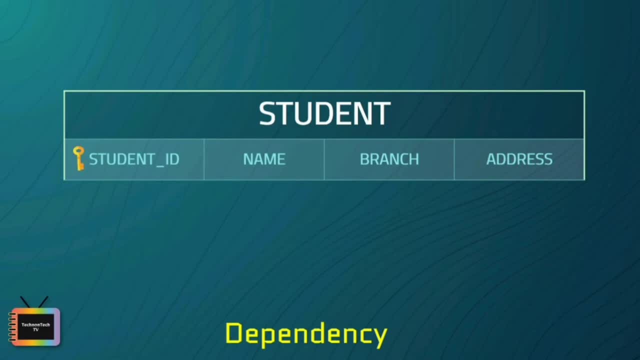 address. In this table, student id is a primary key and will be unique for every row. Hence we can use student id to fetch any row of data from this table, Even for a case where the names are same. if we know the student id, we can easily fetch the correct record. 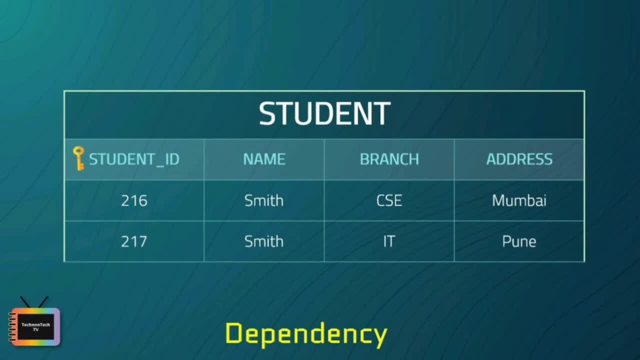 Hence we can say a primary key for a table is the column or a group of columns, or we can say composite key, which can uniquely identify each record in the table. If you don't know the key concept in DBMS, then watch my video. Video link is added in. 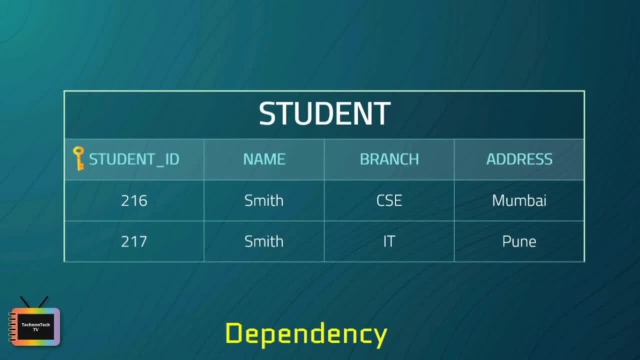 the description box as well as upper right corner of your screen. To understand different normal forms, you should first learn about the key concept. So let's start. First. let's see what is a branch name. So I can ask for branch name of student with student id 216. 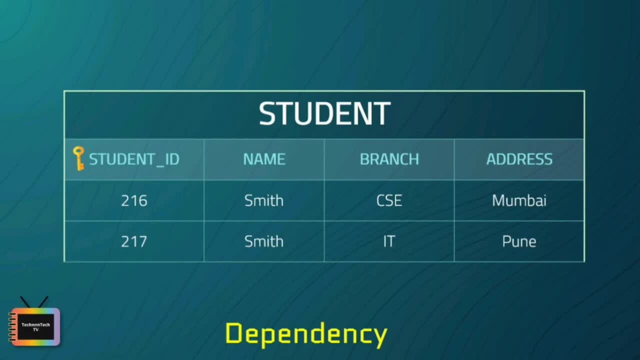 Similarly, if I ask for name of student with student id 216 or 217, I will get it. So all I need is student id and every other column depends on it or can be fetched using it. So this is dependency, and we also call it functional dependency. 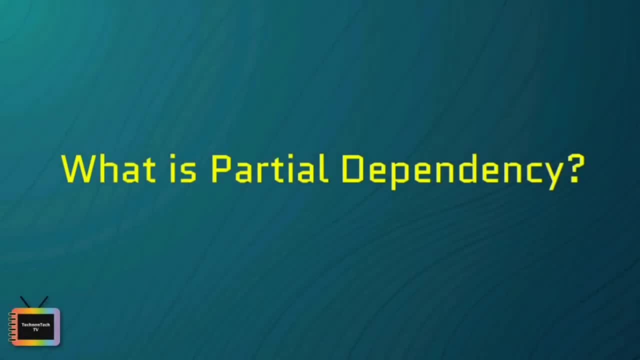 now let's see what is partial dependency. now that we know what the dependency is, we are in a better state to understand what a partial dependency is. so for a simple table, like student, a single column, like student id, can uniquely identify all the records in a table but this. 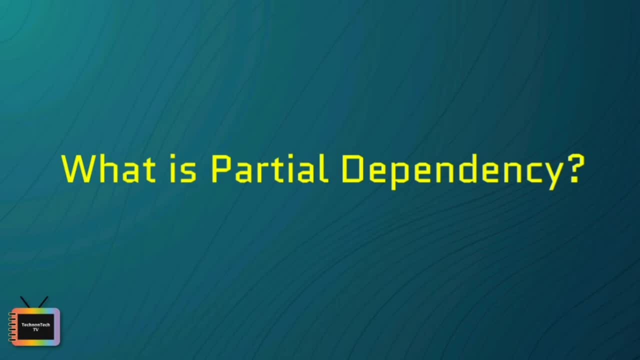 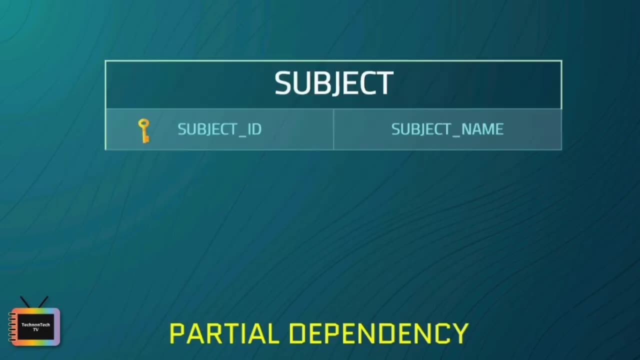 is not true all the time. now let's extend our example to see if more than one column together can act as a primary key. let's create another table for subject which will have subject id and subject name fields, and subject id will be the primary key here. now we have a student. 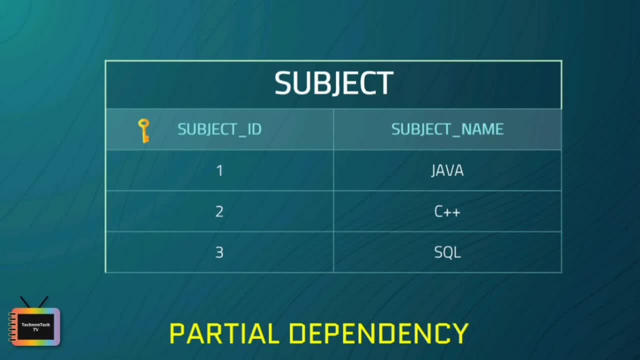 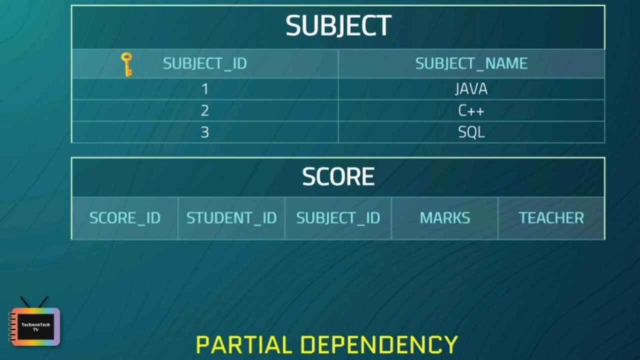 table with student information and another table subject for storing subject information. let's create another table score to store the marks obtained by students in the respective subjects. we will also be saving the name of the teacher who teaches the subject, along with the marks. so in the score table we are saving 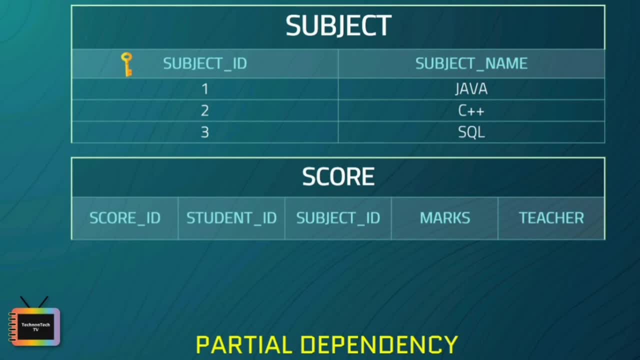 the student id to know which students marks are those, and subject id to know for which subject the marks are for. so together, student id and subject id, forms a candidate key for this table, which can be the primary key. confused right how this combination can be a primary key. 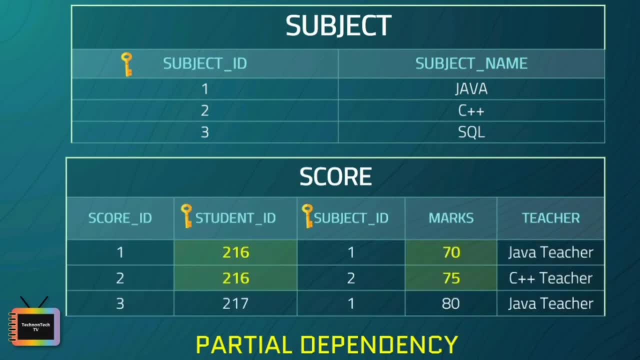 see, if i ask you to get me marks of a student with student id 216, can you get it from this table? no right, because you don't know for which subject, and if i give you only subject id- suppose 1- you would not know for which student. hence we need the student id and subject id to uniquely. 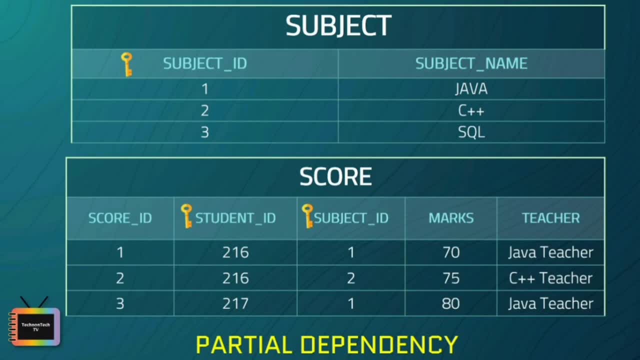 identify any rule. but where is partial dependency here? now, if you look at the table, you'll see that 1 is a zabagat advi. first realize that the student type is student and no, because the all Canadians now must be perfect and also the students need two. 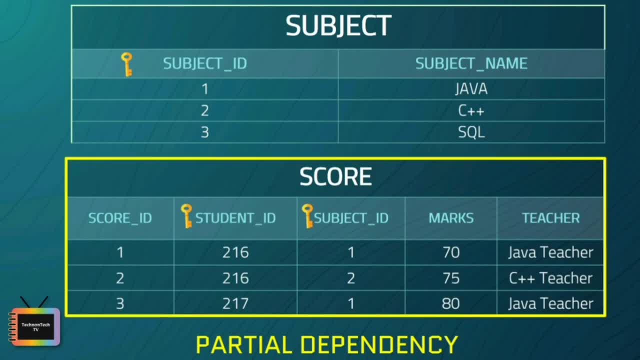 at the score table we have our column names- teacher, which is only depend on the subject. so for Java it's Java teacher, and for C++ it's C++ teacher, and so on. now, as we just discussed that, the primary key for this table is our composition of two columns, which is student ID and subject ID. but the 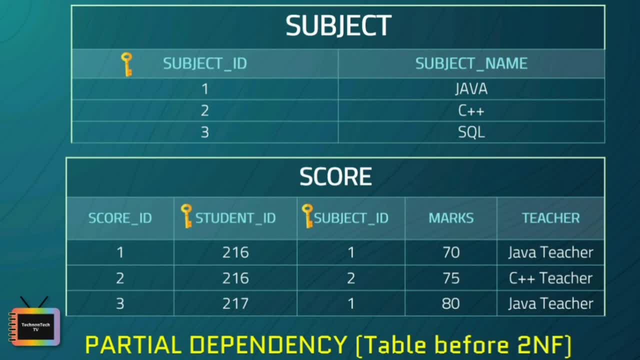 teachers name only depends on subject, hence the subject ID, and has nothing to do with student ID. this is partial dependency, where an attribute in a table depends on only a part of the primary key and not on the whole key. so how to remove partial dependency? there can be different solution for this, but our 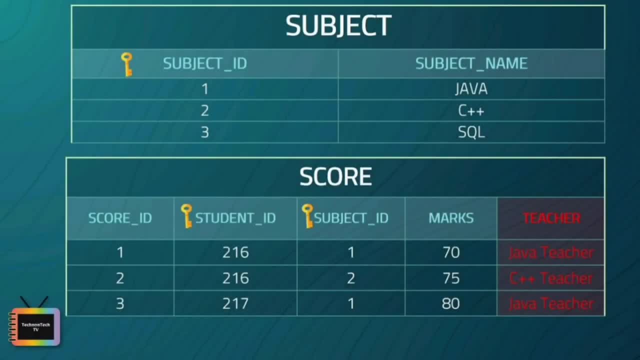 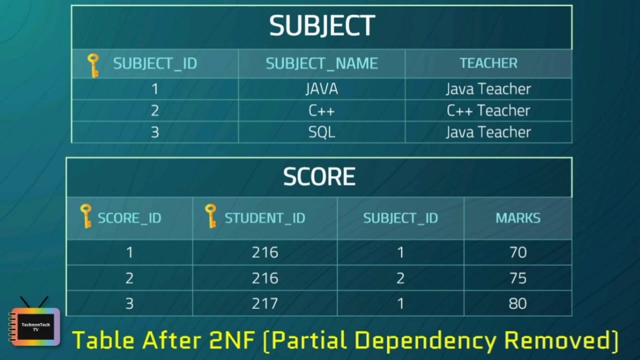 objective is to remove teachers name from score table. the simplest solution is to remove columns teacher from score table and add it to the subject table. hence the subject table will be the subject table and the subject table will be the look like this: and our score table is now in the second normal form, with no 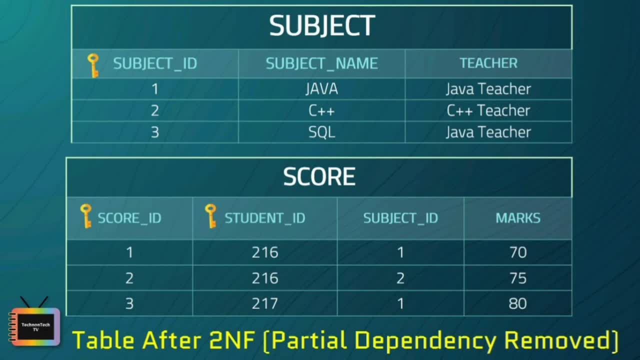 partial dependency. so partial dependency exists when, for a composite primary key, any attribute in the table depends only on a part of the primary key and not on the complete primary key. so to remove partial dependency we can divide the table, remove the attribute which is causing partial dependency and move it. 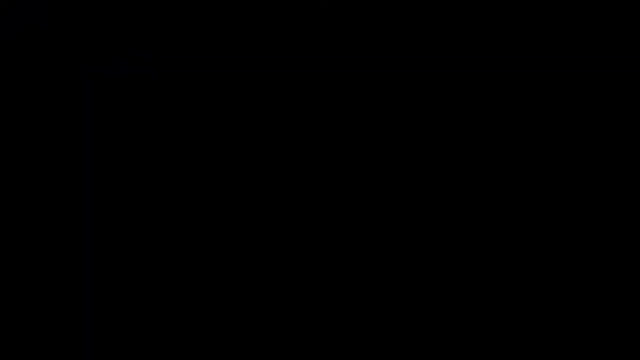 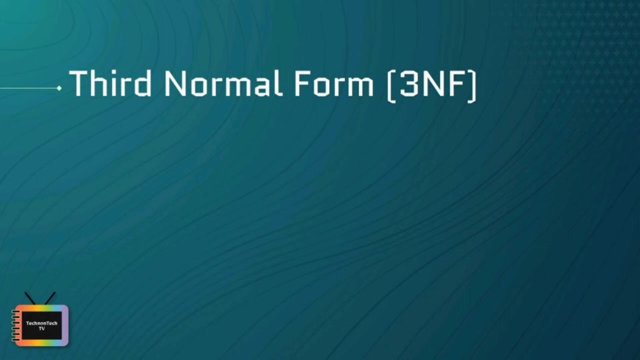 to some other table where it fits in well. so next we have a third normal form, or we can say 3nf. 3nf ensures the referential integrity, reduce the duplication of data, reduce data anomaly and makes the data model more informative. the basic prerequisite for 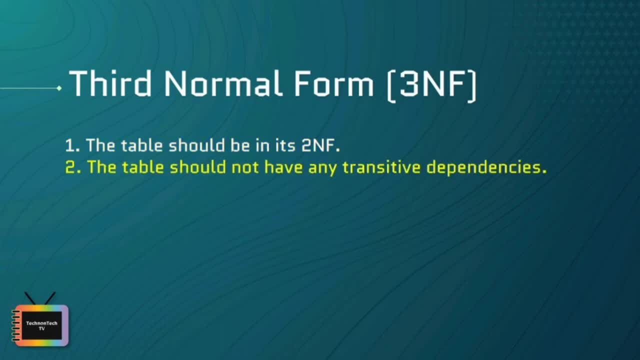 3nf is, the table should be in its 2nf and the table should not have any transitive dependencies. transitive dependency: it occurs due to an indirect relationship within the attributes, when a non prime attribute depends on other non prime attributes rather than depending upon. 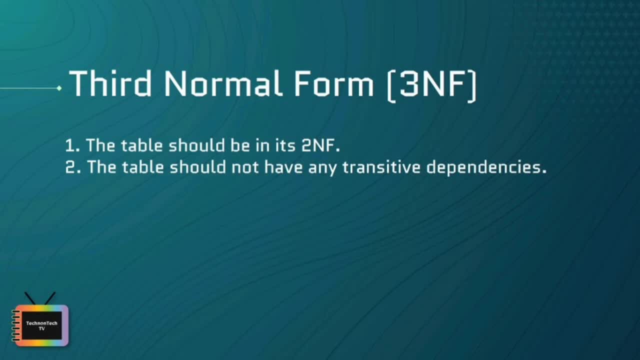 the prime attributes or primary key. so attributes that form a candidate key of a relation, that is, attributes of candidate key, are called prime attributes and rest of the attribute of the relation are non prime. example for the relation: role number, name, city, phone number. role number is a candidate key, hence role number is a 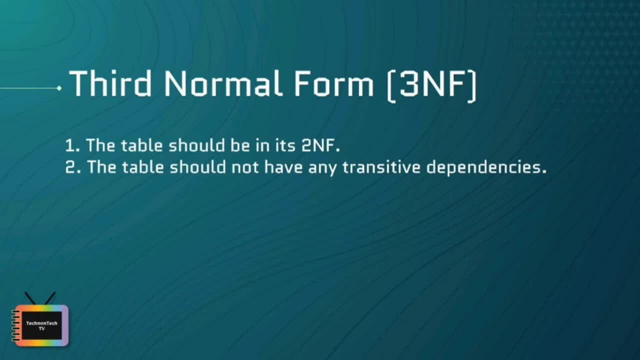 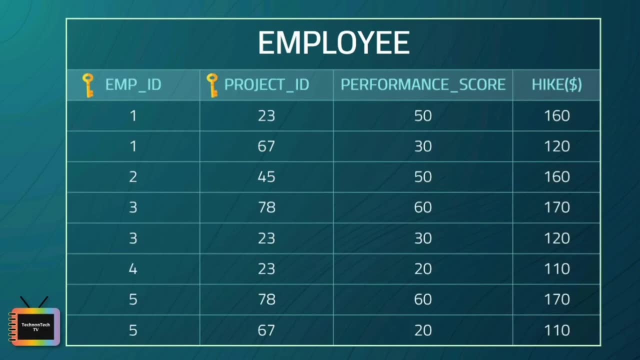 prime attribute and name city, phone number are non prime attributes. consider employee table: in this table employee ID and project ID, both are the primary key, that is composite key, because here one employee is a part of two projects. for example, employee one is a part of two projects, that is 23 and 67, and also we 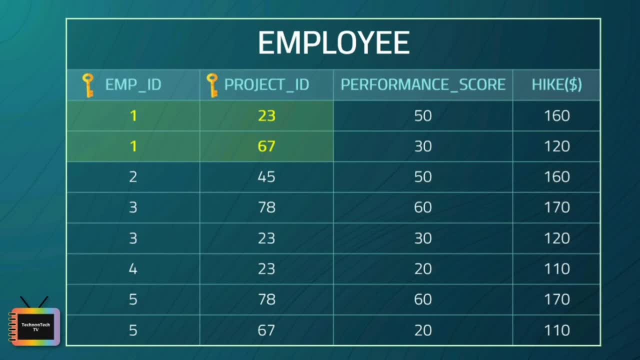 cannot alone assign project ID as a primary key, because we also need employee information uniquely so that we can get the performance score of a particular employee. that's why employee ID and project ID both are the composite key here. so for this table the performance score depends on both employee and project that he is. 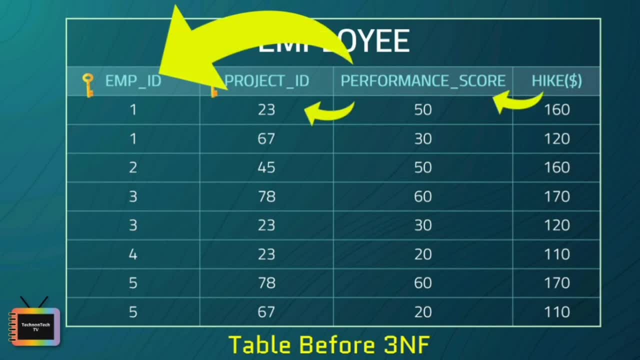 associated. but the last column, height, depends on performance score. the height changes with performance and here the attribute performance score is not a primary key. this forms our transitive dependency. so to eliminate the transitive dependency created and to satisfy the 3 NF, the table is broken. 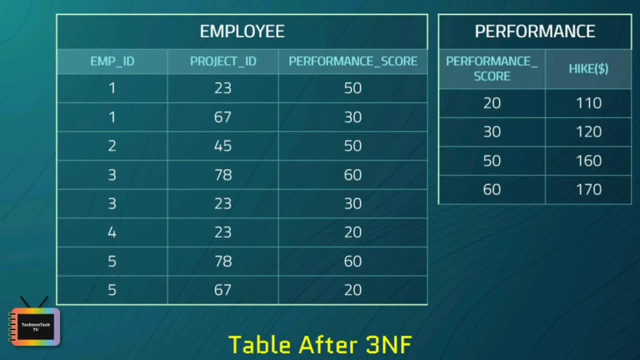 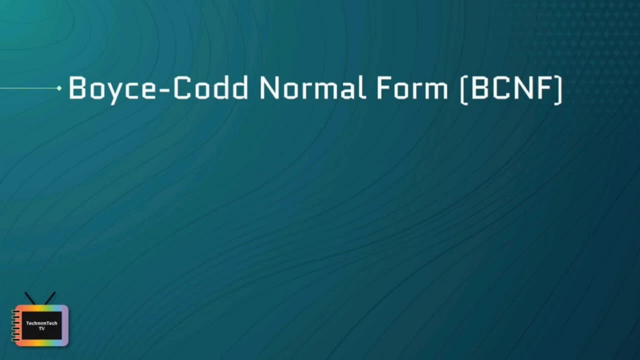 down into two tables, that is, employee table and performance table. now it satisfy 3 NF. we have a Boy Squad normal form or we can say BCNF. BCNF is an extension to the third normal form and it is also known as 3.5 normal form for 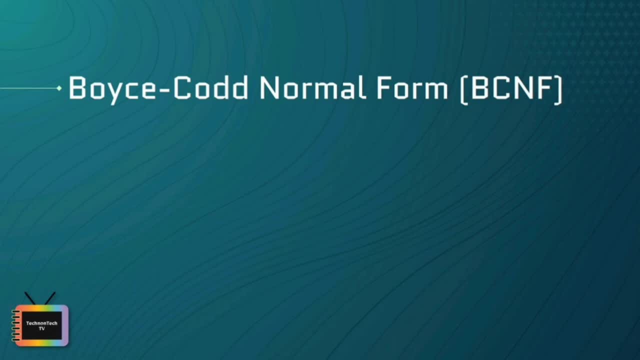 a table to satisfy BCNF. it should satisfy these two conditions. it should be in the third normal form and for an dependency, B depend on a, they should be a super key. the second point sounds a bit tricky, right. in simple words it means that for our dependency, that is, B depends on a, he cannot be a non prime. 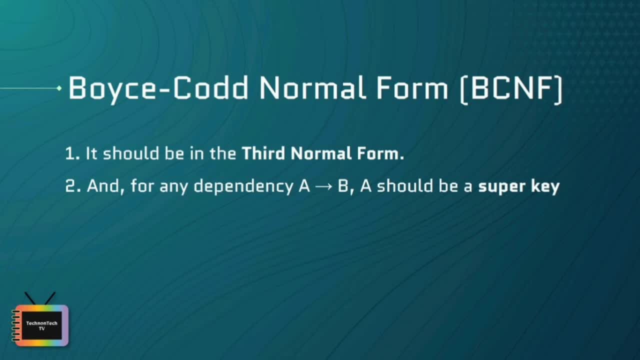 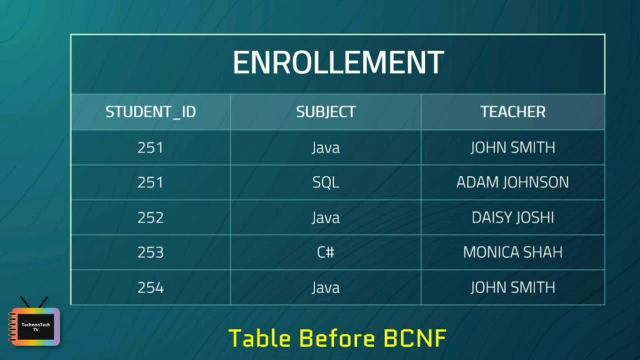 attribute if B is a prime attribute. so let's see the example. so we have a college enrollment table with the column student ID, subject and teacher. now in this table one student can enroll for multiple subject. for example, student with student ID 251 has opted for subject Java and SQL. so for each 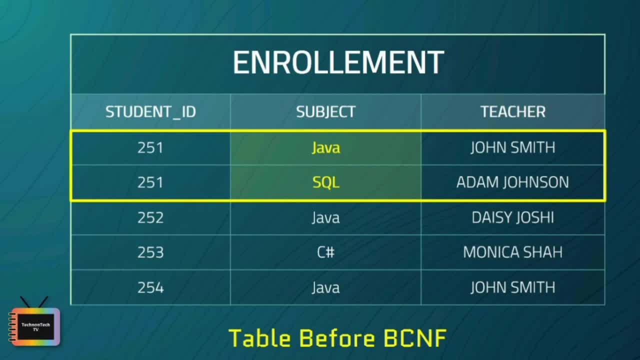 subject our teacher is assigned to the student and there can be multiple teachers teaching one subject, like we have for Java. so what do you think should be the primary key? well, in this table, student ID, subject, together form the primary key. using student id and subject, we can find all the columns of the table. one more important point to 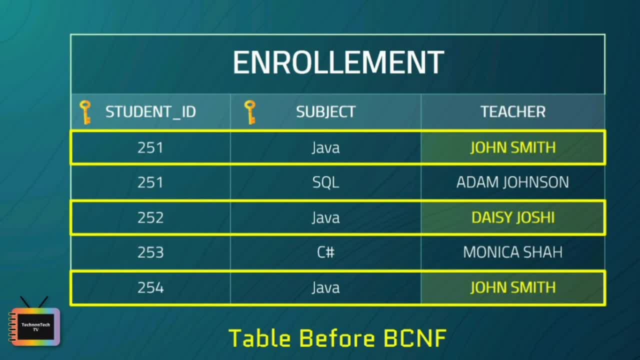 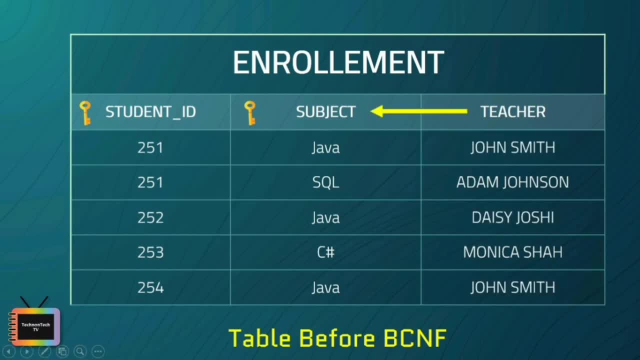 note here is: one teacher teaches only one subject, but one subject may have two different teachers. hence there is a dependency between subject and teacher here, where subject depends on the teacher name. this table satisfy the one normal form because all the values are atomic, column names are unique and all the values stored in a particular columns are of same domain. this table. 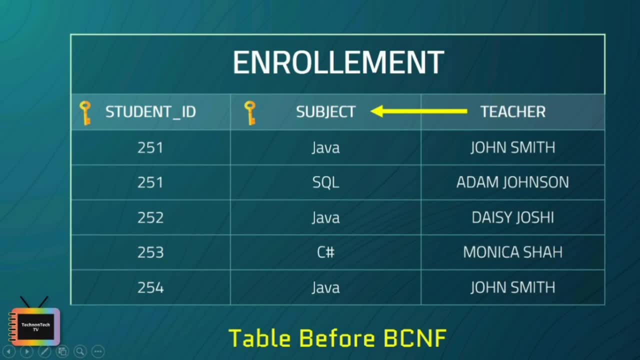 also satisfy the second normal form, as there is no partial dependency and there is no transitive dependency. hence the table also satisfies the third normal form. but this table is not in bc nf. why this table is not in bcnf? so in this table, student id, subject, form, primary key, which means: 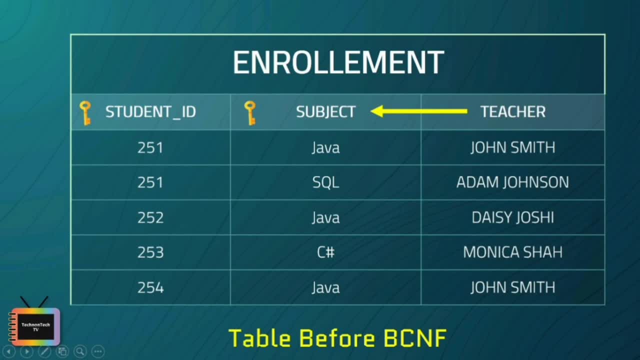 subject column is not in bc nf, so in this table student id, subject form primary key is not in bc a prime attribute. but there is one more dependency, that is, the subject is depend on teacher and while subject is a prime attribute, teacher is a non-prime attribute which is not allowed by bcnf. so how to 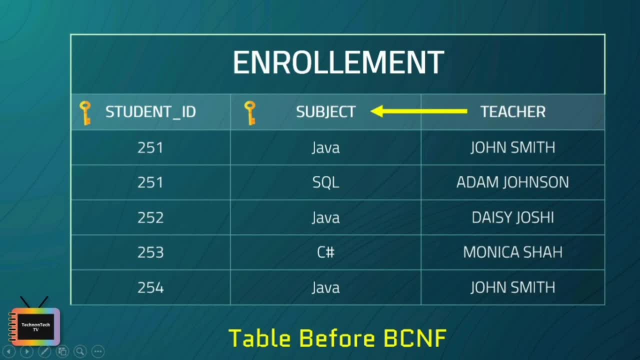 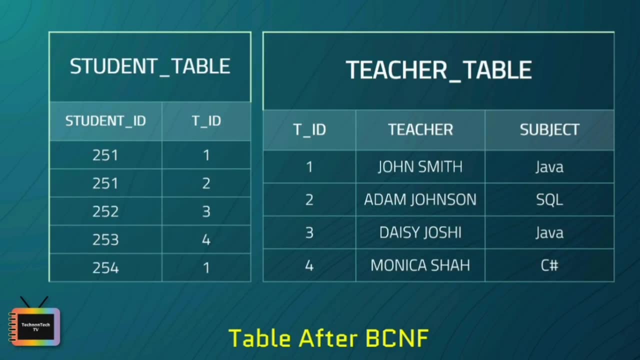 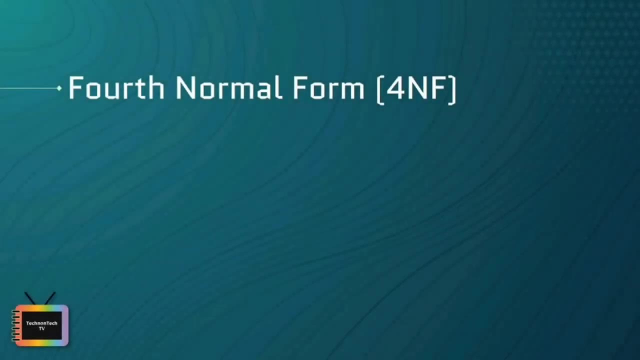 satisfy bcnf. to make this relation satisfy bcnf, we will decompose this table into two tables: student table and teacher table. and now this relation satisfy boy square normal form or bcnf. next we have a fourth normal form, or we can say 4nf. our relation will be in 4nf if it is. 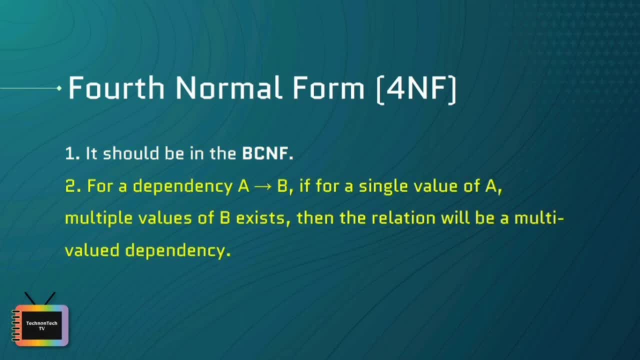 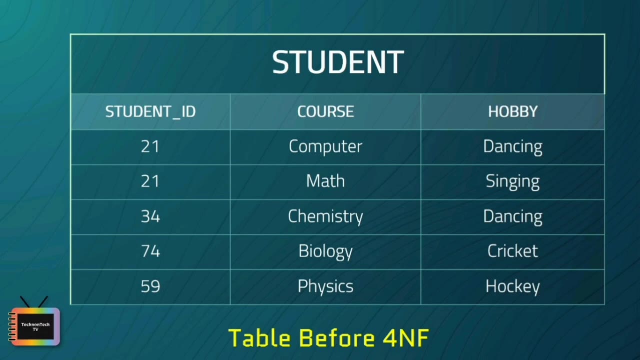 in bcnf and has no multi-valued dependency. for a dependency, b depend on a. if for a single value of a, multiple values of b exist, then the relation will be a multi-valued dependency. for example, this student table is in 3nf, but the course and hobby are two independent entity. hence there is 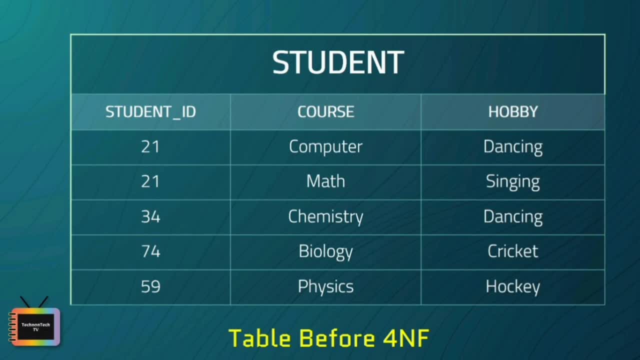 no relationship between course and hobby in the student relation. a student with student id 21 contains two courses- computer and math- and two hobbies, that is, dancing and singing. so there is a multi-valued dependency on student id which leads to unnecessary repetition of data. well, the 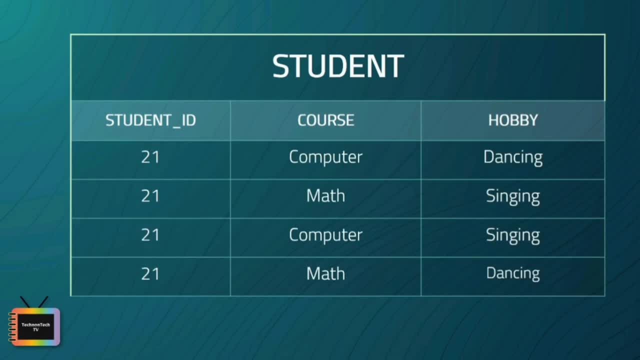 two records for student with student id 21 are two courses- computer and math- and two hobbies. that is, student id 21 will give rise to two more records, as shown here, because for one student two hobbies exist. hence, along with both the courses, these hobbies should be specified, and in this table, 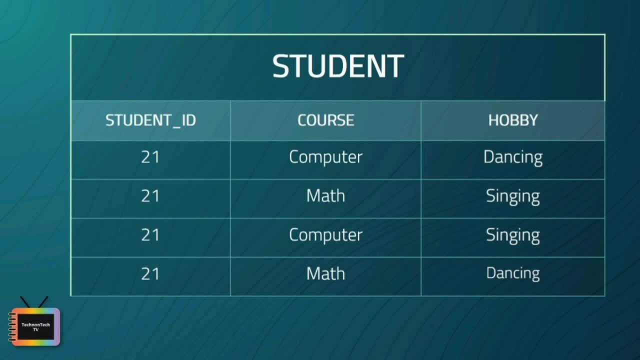 there is no relationship between the columns, course and hobby. they are independent of each other. so there is multi-value dependency which leads to unnecessary repetition of data and other anomalies as well. so how to satisfy bcnf? to make this relation satisfy boy, square, normal form or bcnf? 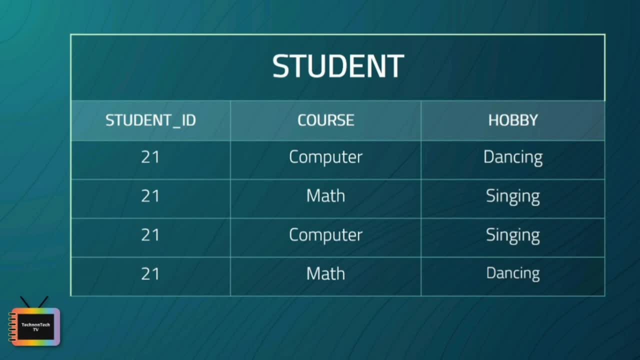 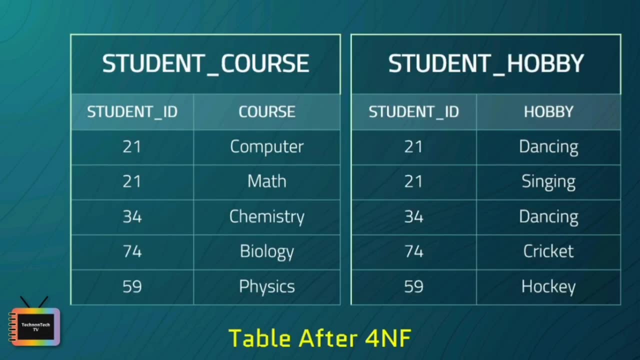 satisfy fourth normal form. so to make this relation satisfy the fourth normal form, we can decompose this table into two table that is, student course and student hobby. and now this relation satisfy fourth nf. so that's it for this video. i hope you learned something new today. do share this. 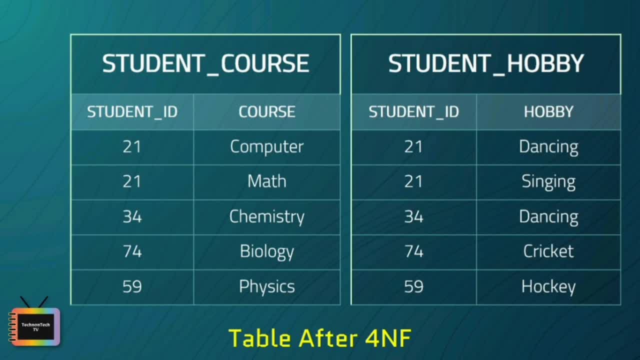 video with your friends to spread the knowledge. if you have any questions, let me know in the comment section, and if you want to see more videos like this in the future, please like and subscribe, and don't forget to hit the bell icon so you don't miss out on any of my future videos. thank you, and i will. see you in the next video. bye.